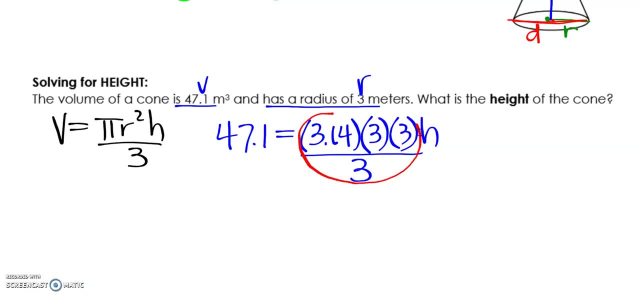 to do is go ahead and multiply pi times three times three divided by three. So 47.1 is equal to. when I calculate that value, I get 9.42 times h. We're going to bring h down into the next step. 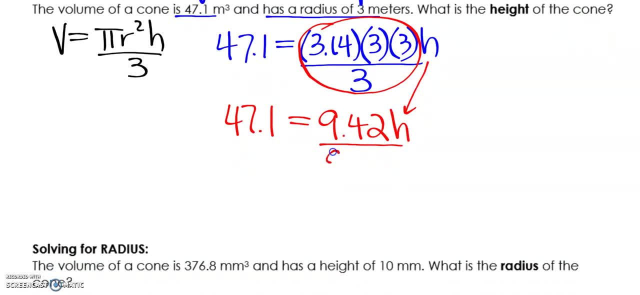 of our work and divide. now We're going to divide by 9.42.. First operation of multiplying 9.42 times h would be to divide by 9.42.. So we're going to do that on both sides of the equal sign and our height is going to equal five meters. And that measurement 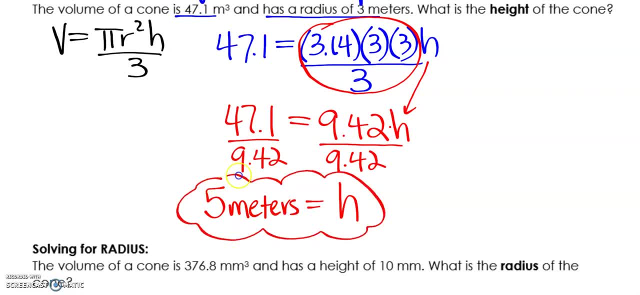 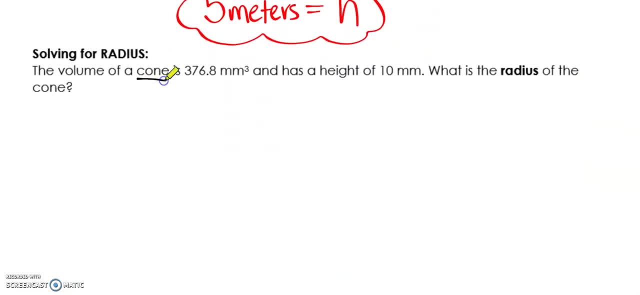 is not cubed, because it's just the height measurement, and that is one dimension. Let's go to the next example, where we solve for radius. Okay, so we're going to write our formula again. We're solving for the radius of a cone. So volume equals pi r squared times height divided by three. 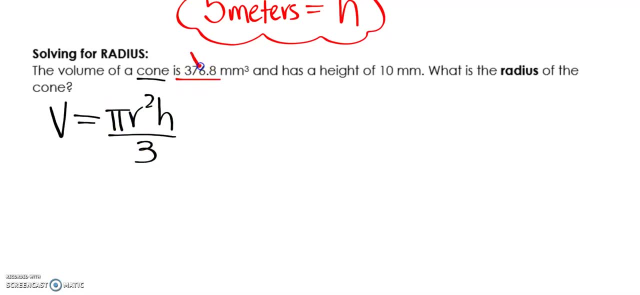 We're going to substitute 376.8 in for volume, So that's 376.8 equals pi, which is 3.14 times the radius squared, which we don't know. So we're going to put that down as r squared. and then the height. 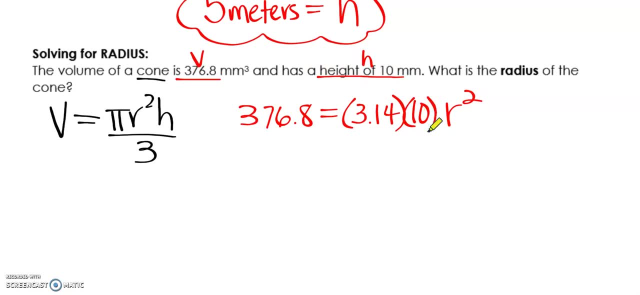 is 10.. So we're going to substitute. It's okay if I write the 10 before the r squared, but order doesn't matter when we are multiplying And then finally divide by three. So the first thing I would like for you to do is plug in 3.14 times pi squared, times the radius squared. So that's. 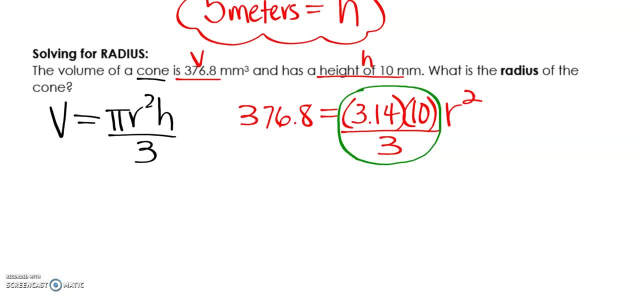 10 and divide that value by three, That does give you a repeating decimal: It's 10.46666666.. We're going to round that to 467.. Okay, the more you can carry out these three digits of this number, 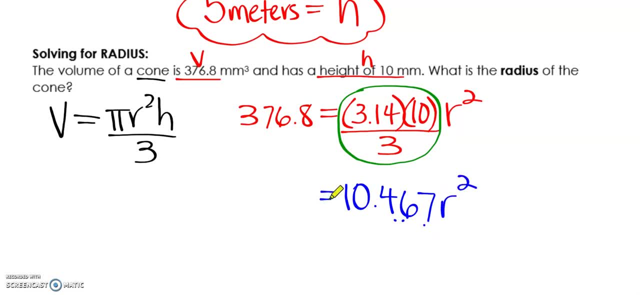 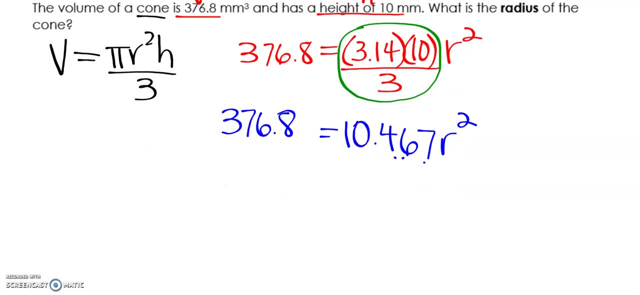 the more accurate your answer is going to be That repeating decimal kind of makes things a little bit different. All right, 376.8 comes down to the next step of the problem. So the next thing we'll do is divide by 10.467, just like we did when we solved for r squared. So we're going to 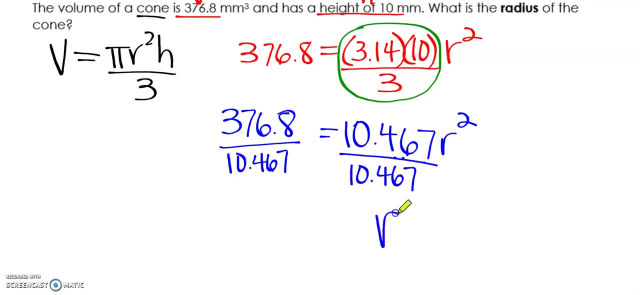